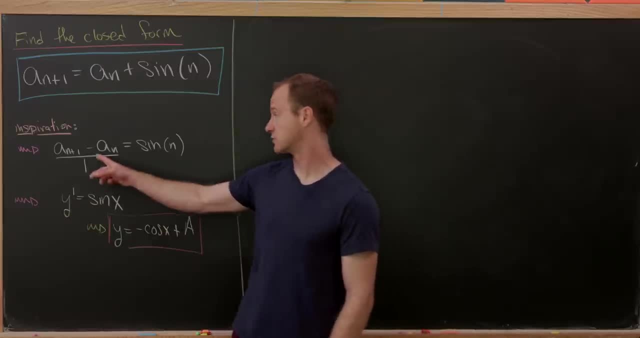 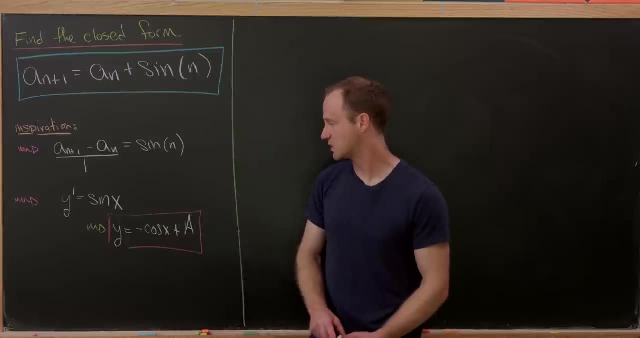 Y. y prime equals sine of x, because we've got derivative over here and then sine over here. but that's easy to solve. just by taking the anti-derivative we'll get minus cosine of x, plus some constant a. so now let's take inspiration from this and form maybe a first guess for our. 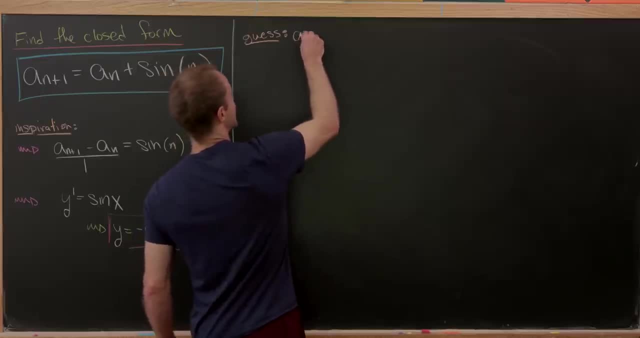 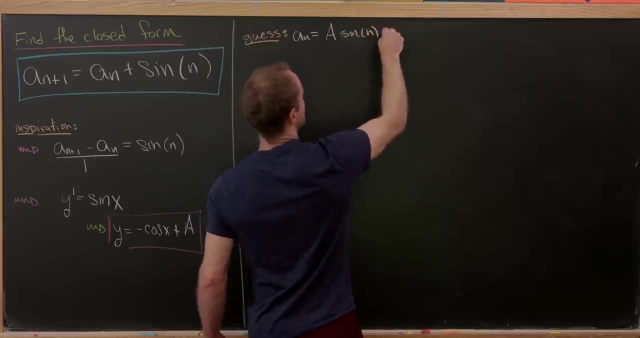 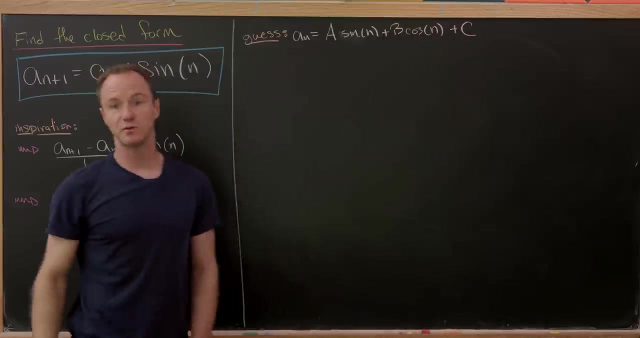 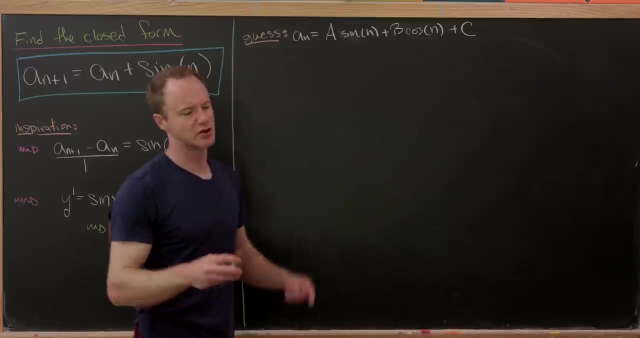 solution, and that guess will be to set a sub n equal to some constant a times sine of n, plus some constant b times cosine of n, and then, just for good measure, we'll say some constant c, because we expect, you know, there to be a constant, basically with respect to integration. 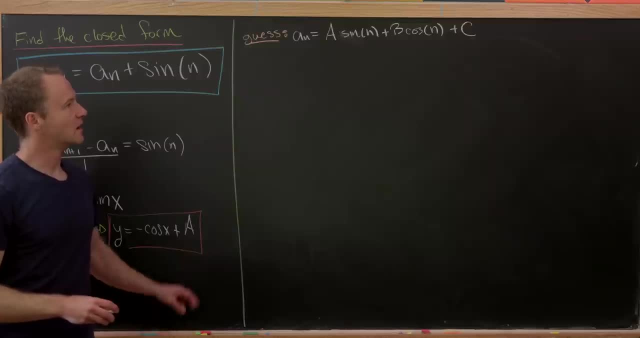 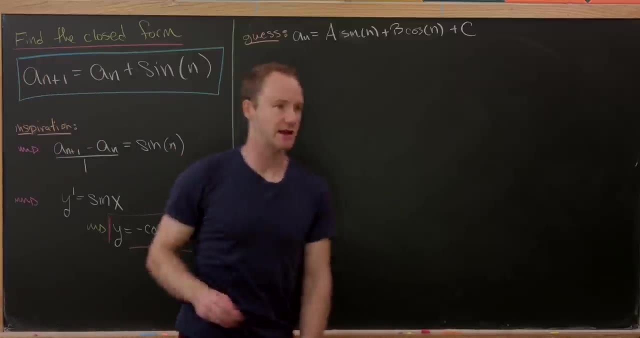 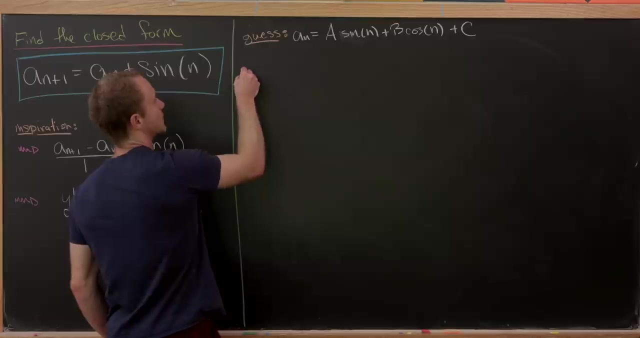 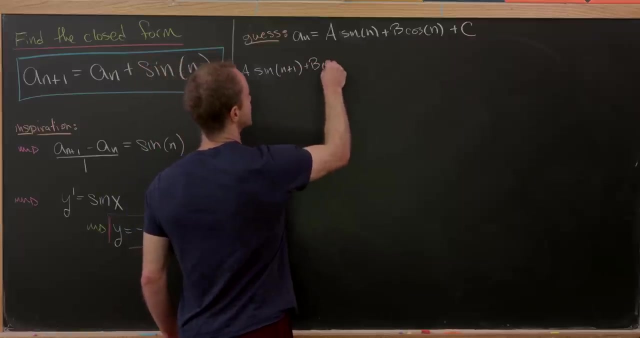 or a constant of integration built into this, okay. so now let's plug this into our- well, it's called the difference equation, this thing right here. Okay. so let's do a n plus one first. So notice, a n plus one is a times sine of n plus one plus b times cosine of. 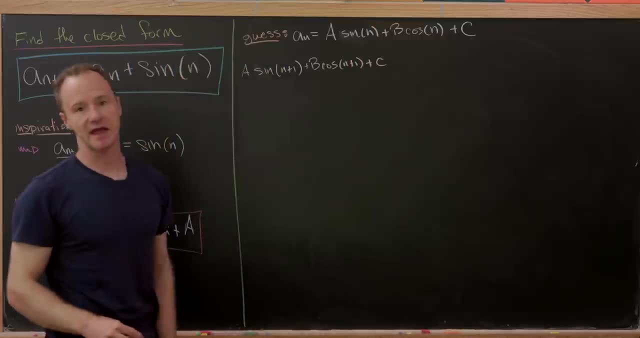 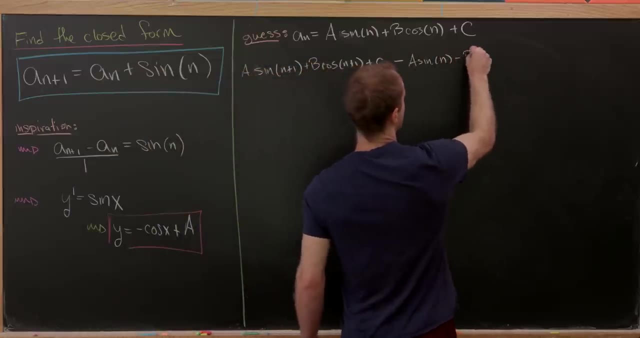 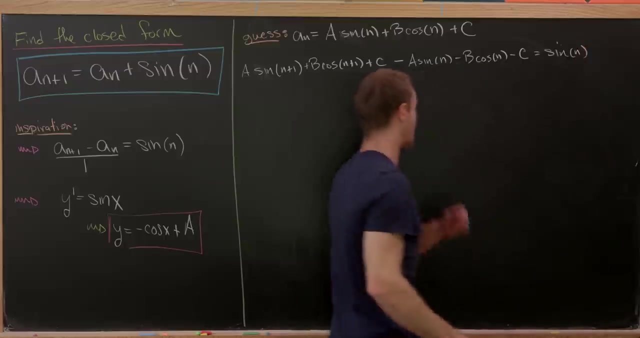 n plus one plus c. So, like I said, that's our a? n plus one, and then from that we need to subtract a- n, so that'll be a sine of n minus b, cosine minus c, and this all needs to be equal to sine of n. 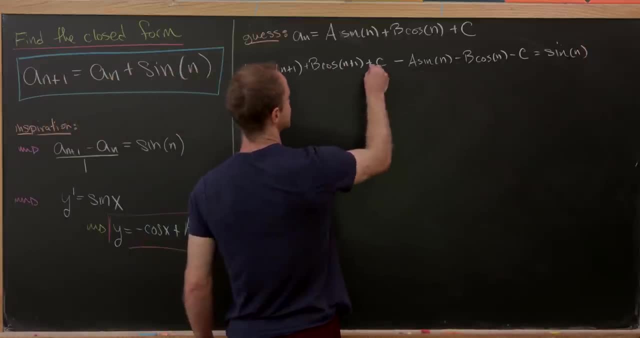 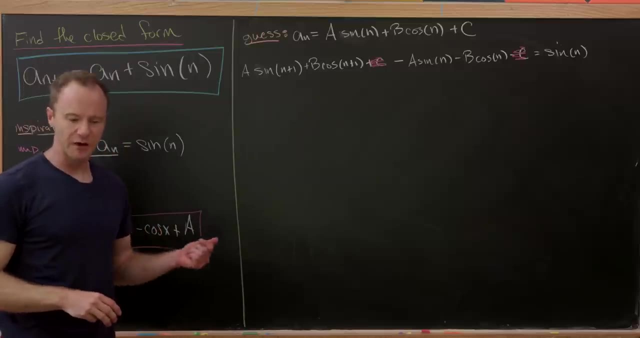 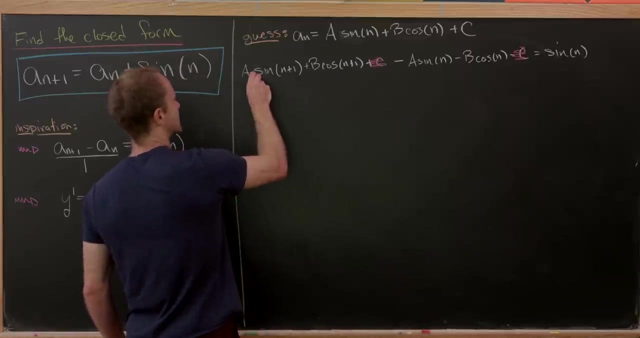 Well, let's quickly notice that these c's cancel. They cancel immediately, which means really the c is allowed to be anything we want, which I think we probably expected to be true. So next up we look at these kind of odd terms out, And I would say the odd terms out are the sine of n plus one and the cosine of n plus one, and we 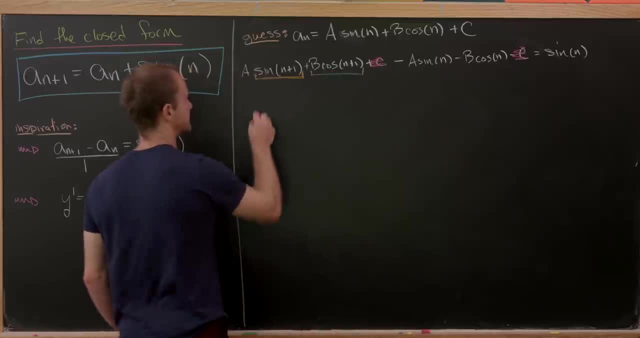 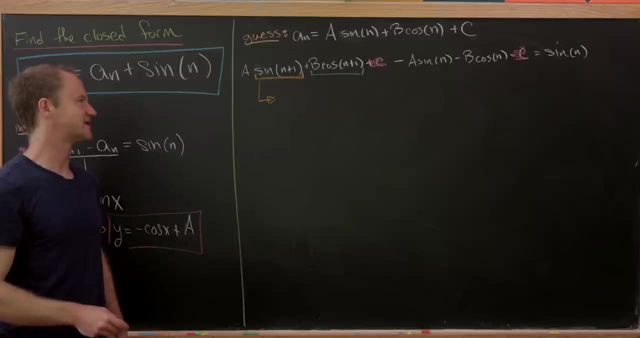 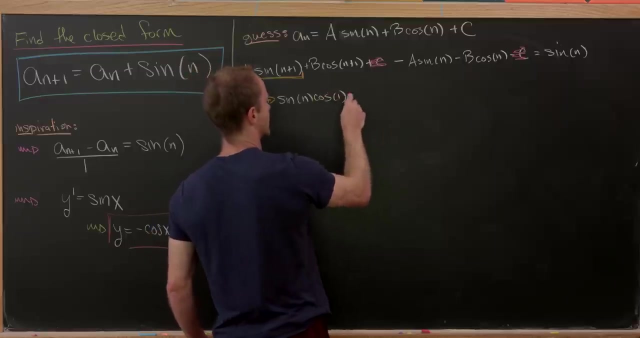 think to ourselves: well, what can we do with these? But there are some nice formulas which are. but there are some nice sum angle formulas that will help us simplify these, and that would be: sine of n times cosine of one, plus sine of one times cosine of n. So again that's. 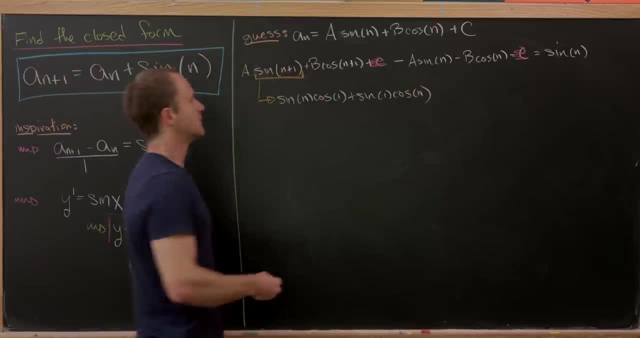 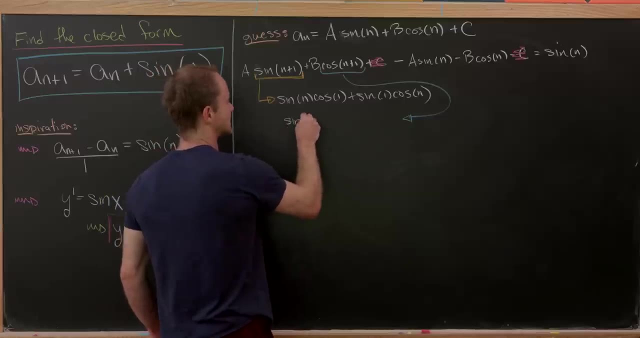 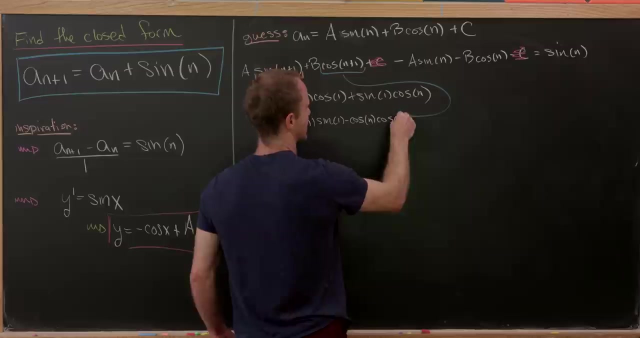 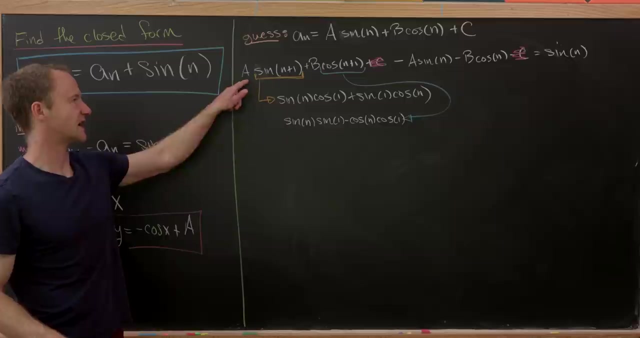 a well-known sum angle formula for sine, But there's also one for cosine, and that's also pretty nice. So what would that leave us with? Well, it would be sine of n times sine of one minus cosine of n times cosine of one. Okay, good, So now let's plug those into, well, the place where we see sine. 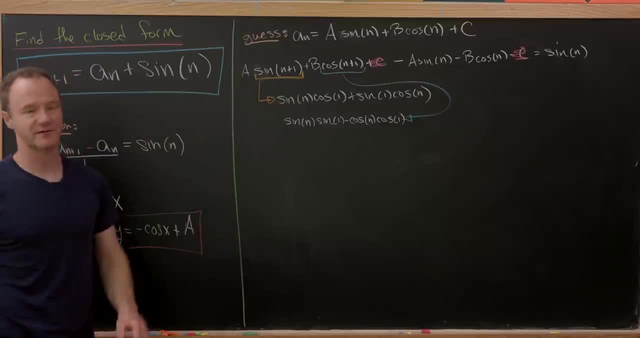 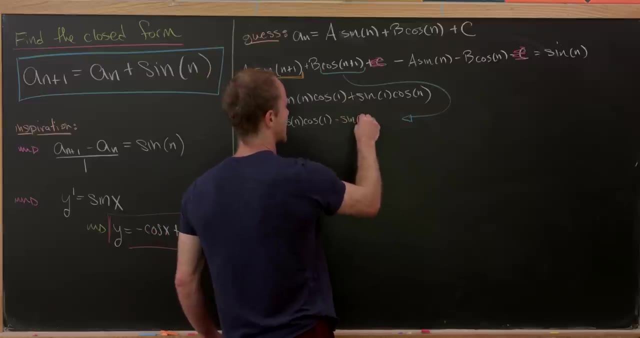 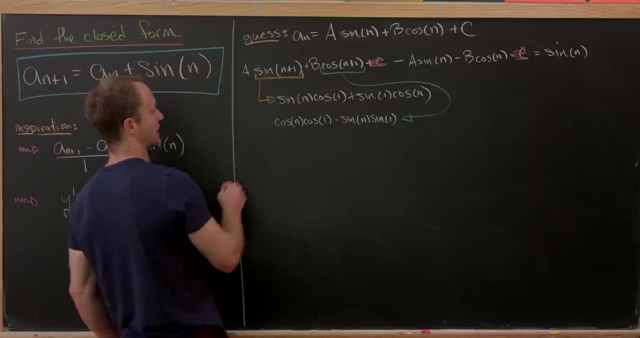 of n plus one and cosine of n plus one, and see what sort of simplification occurs. So this gives us cosine of n times cosine of one minus sine of n times sine of one. Okay, good, And now let's expand this whole thing out, So we'll have a times cosine of one times sine of n. 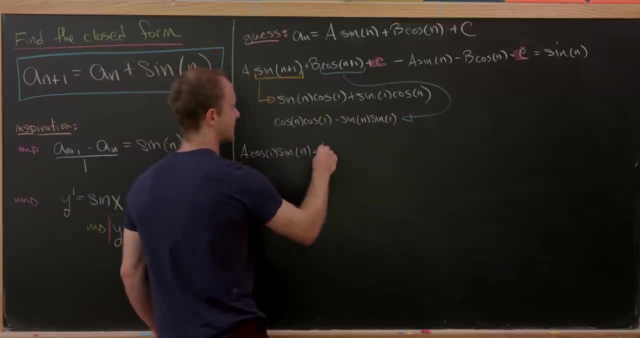 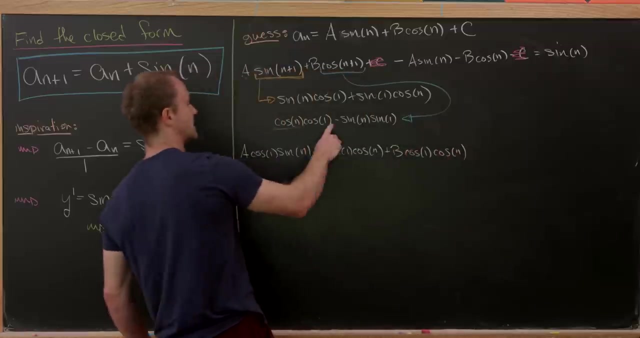 That's a multiplying through to this term, And then plus a times sine of one times cosine of n, A multiplying through to this term, And then we'll have plus b times cosine of one times cosine of n, That's b multiplying through to this, minus b times sine of. 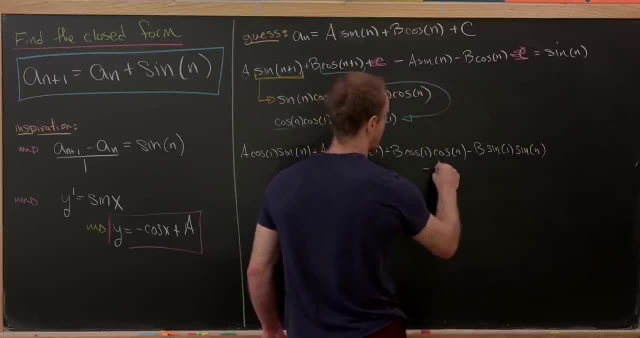 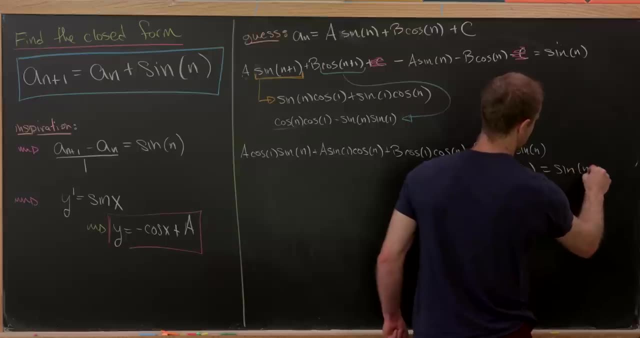 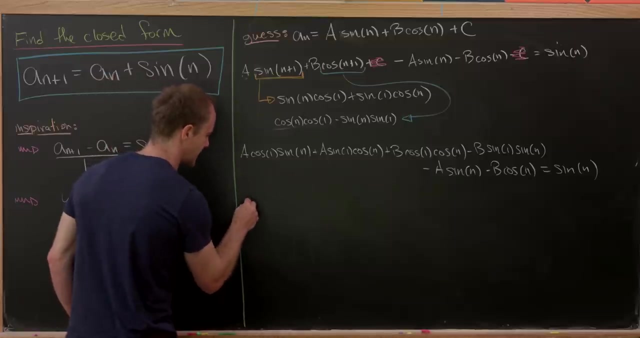 one times sine of n, And then finally, minus a times sine of n, minus b times cosine of n equals sine of n. So there's a lot going on there. But now we're going to use the fact that the sine function and the cosine function are linearly independent. But that's just a fancy way of saying. 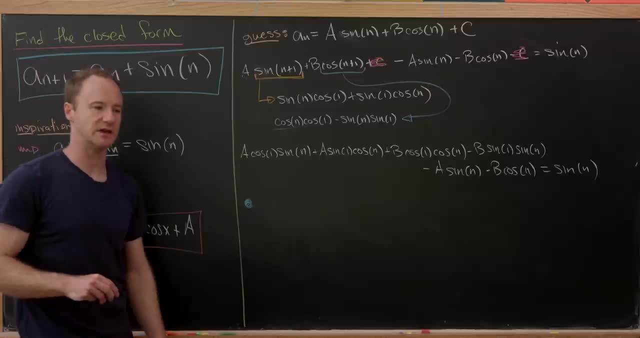 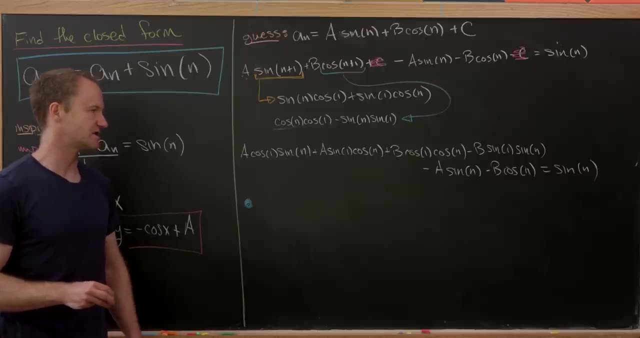 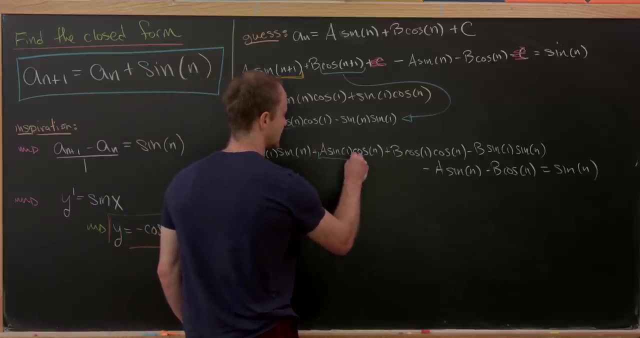 that. So let's take this equation right here that has two unknowns, a and b, and pull it apart into two equations with two unknowns by extracting the coefficients of cosine of n and sine of n. So let's start with the coefficients of cosine of n. So here we have a times sine of one. Here we have 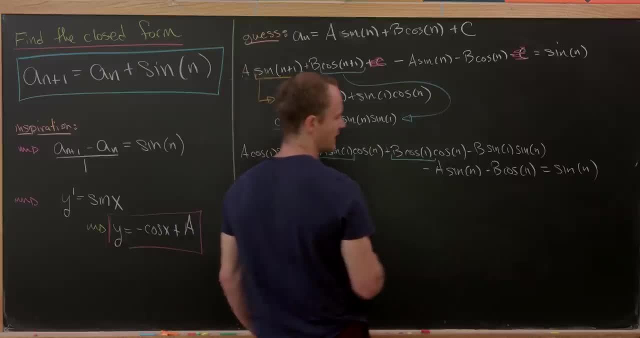 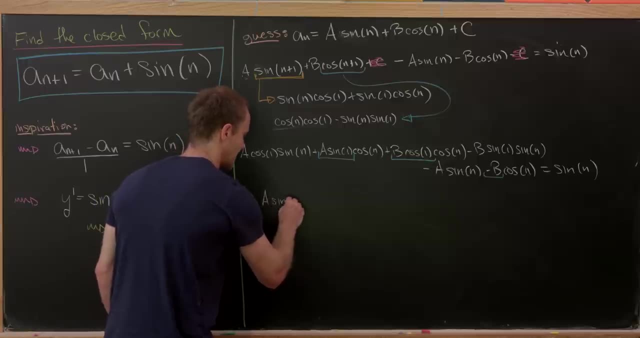 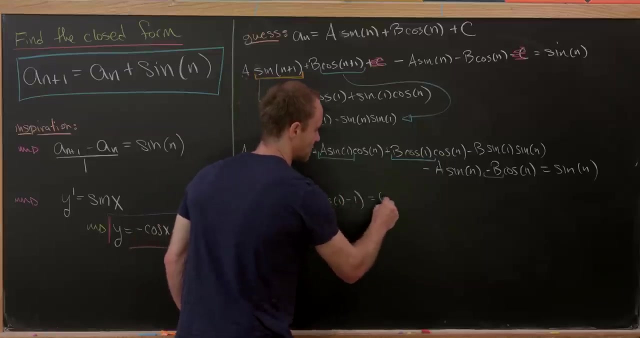 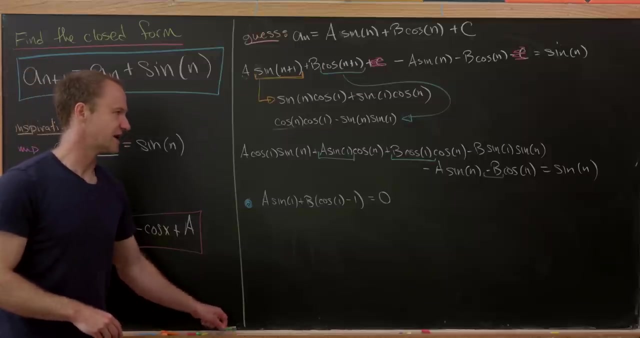 b times cosine of one, And then finally, here we have minus b, So that'll leave us with a times sine of one, And then plus b times cosine of one. minus one equals zero, Because I guess I should say there's no cosines on the right hand side. Now let's do the same thing with the coefficients. 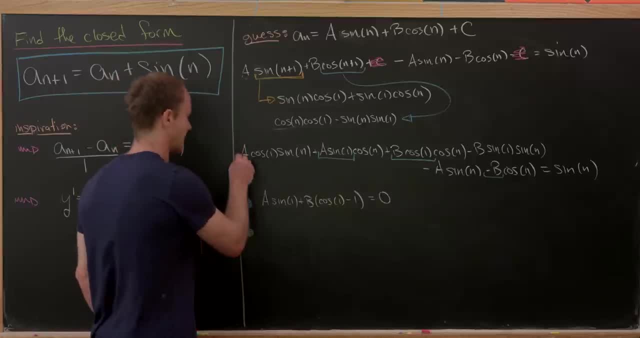 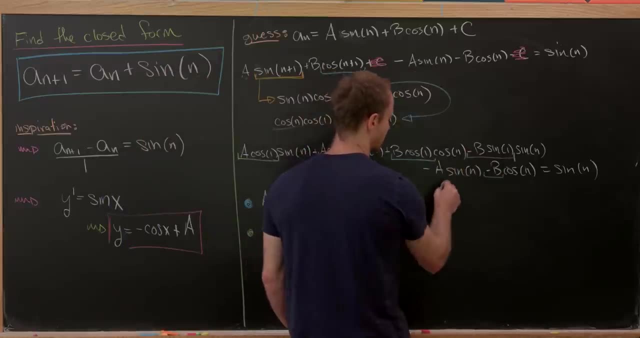 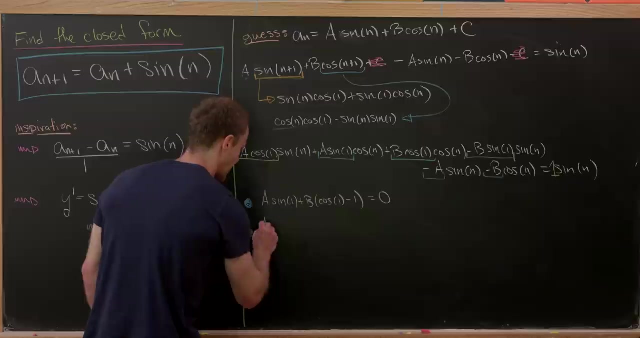 of sine of n. So let's see, We have a times cosine of one right here, Then we have negative b times sine of one, And then we have minus a right here And then I guess we have the number of cosine of one over here. So that'll leave us with a times the quantity cosine of one minus one from the first. 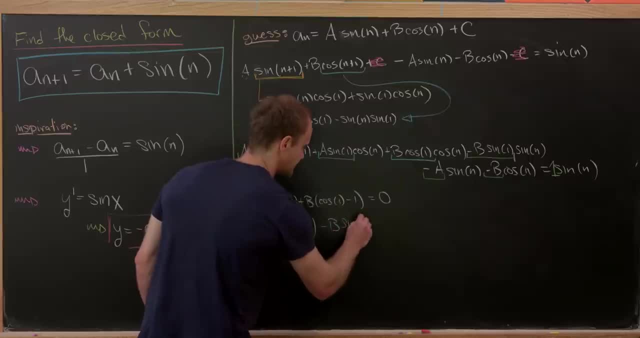 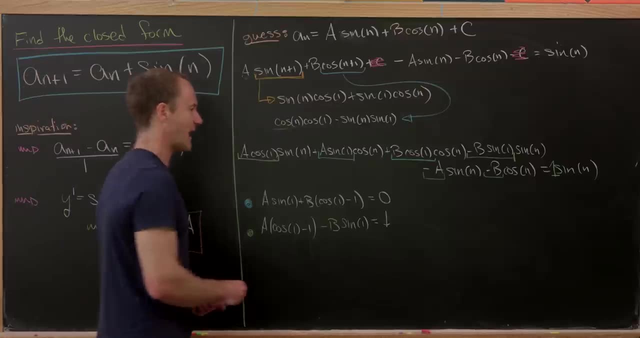 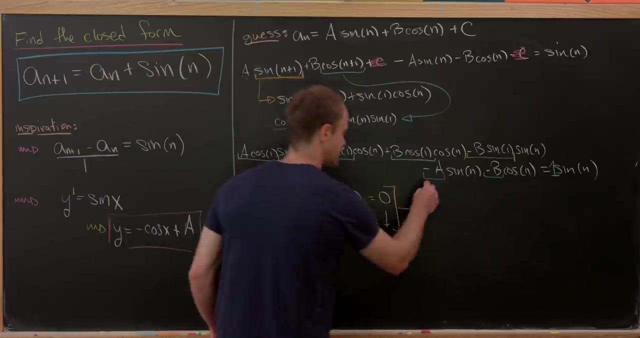 two terms, And then minus b times sine of one, And that's going to be equal to one. now, Okay, But now we're going to pass this system of equations to a matrix vector equation. It's just going to make everything a little bit simpler to solve. So this is equivalent to the following matrix vector: 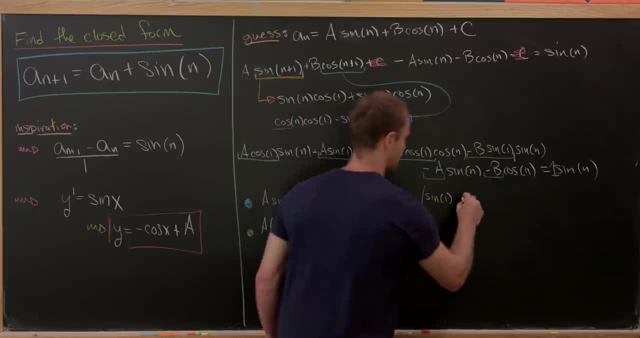 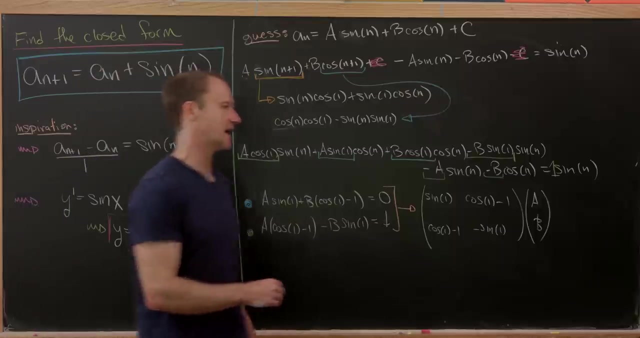 equation. So we'll have a sine of one And then we'll have a cosine of one, And then we'll have a cosine of one up here And then a cosine one minus one here, A cosine one minus one here, And then a minus sine one here. So this multiplied into the vector of coefficients a and b must be: 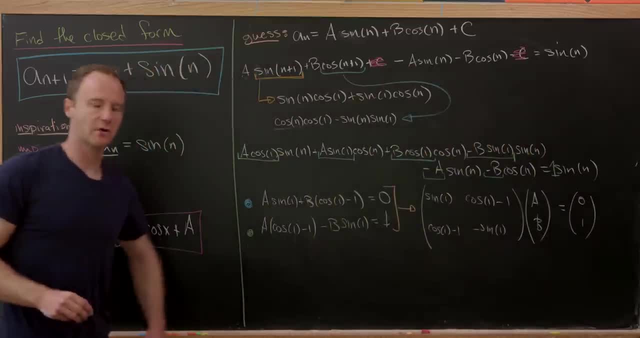 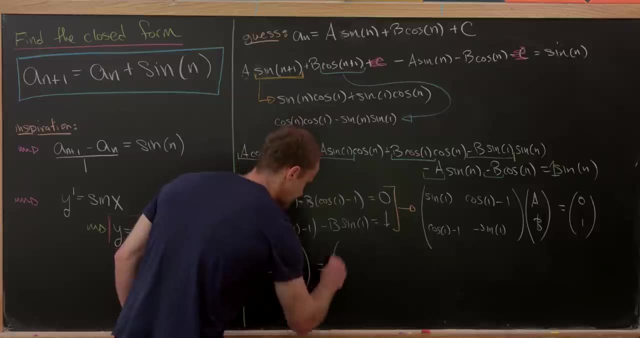 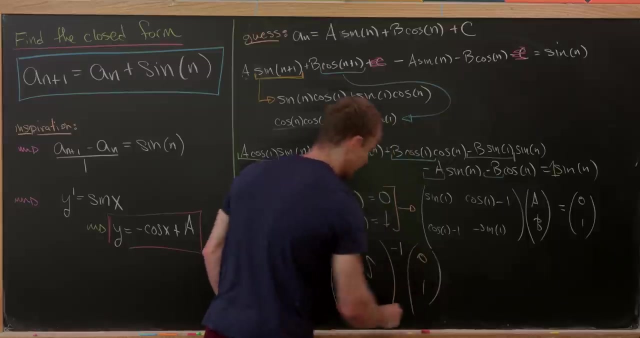 equal to zero one. Okay, Great, But notice that allows us to solve for this vector of coefficients fairly easily. So it'll be this big matrix right here, And then we'll have a cosine of one minus one over here, Which maybe I won't enter in Inverse times: the vector zero one. Okay, So let's. 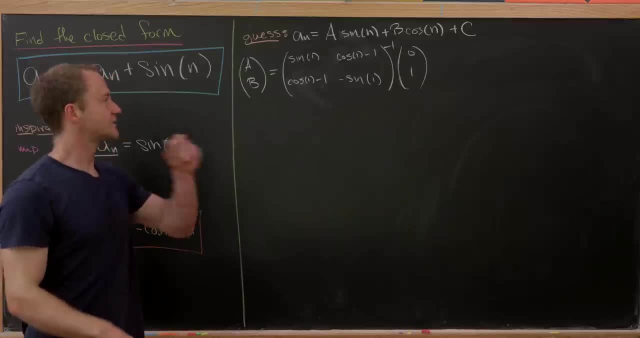 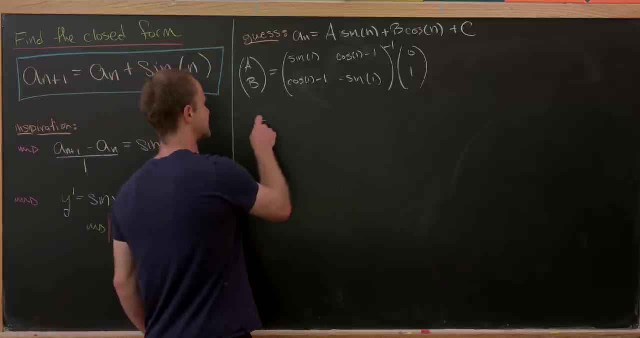 maybe bring that to the top and do the last couple of steps. Okay, So this is where we left ourselves off, And now we're ready to finish it off. So let's start by taking the inverse of this matrix. But since it's a two by two matrix, there's an easy way to do that, So we'll have one over. 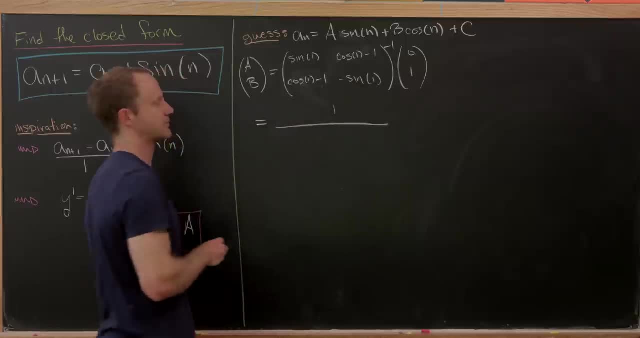 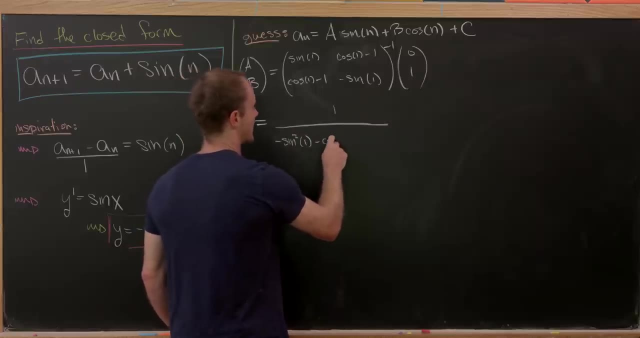 its determinant, Which is the product of the diagonals minus the product of the off diagonals. So that'll leave us with negative sine of one minus one, And then we'll have a cosine of one minus sine squared of one, And then we'll have minus cosine squared of one plus two cosine of one. 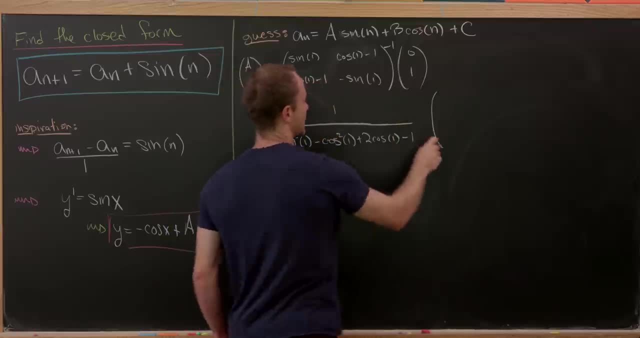 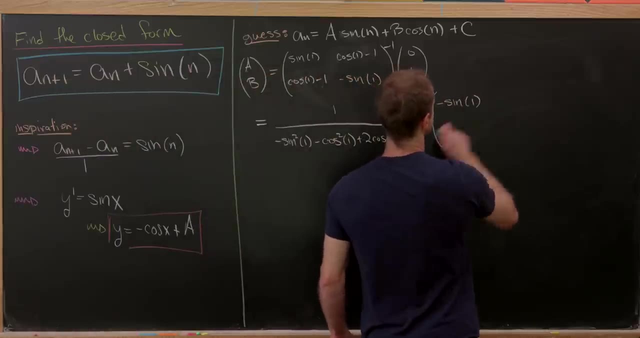 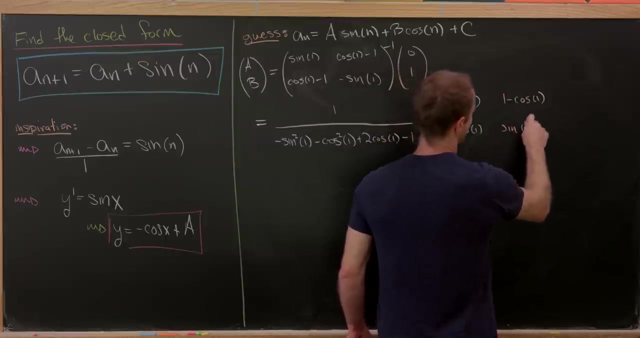 And then minus one. And then how do we get the rest of it? Well, we build the matrix by swapping the diagonals and negating the off diagonal. So that'll be minus sine of one here, One minus cosine of one here and here, And a positive sine of one here, And that's multiplying into